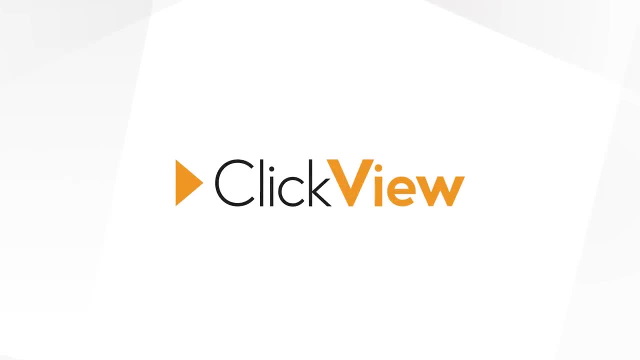 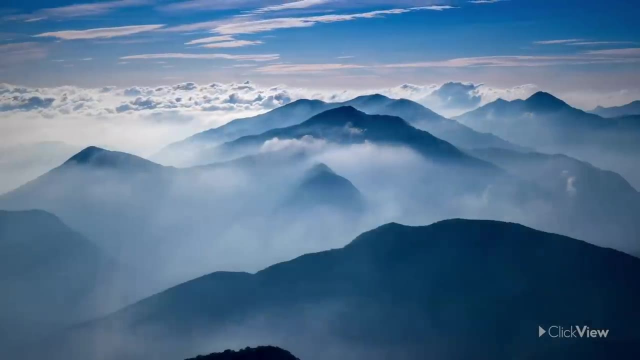 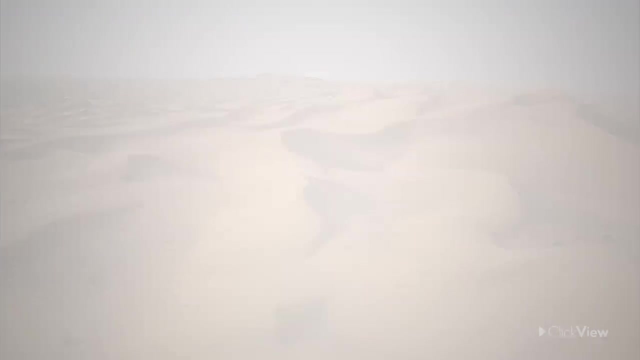 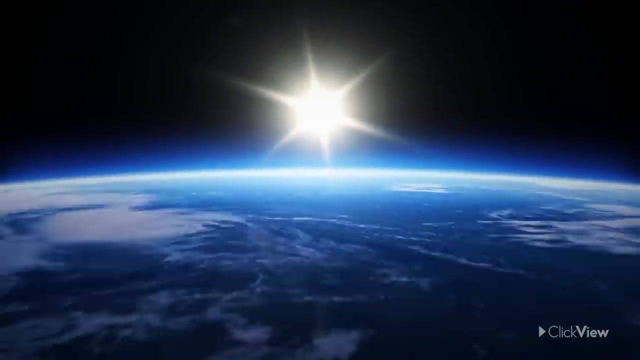 Oceans, mountains and continents. These are just some of the features that make up the world that we live in. The Earth's surface makes up only a tiny fraction of our planet, which we call the crust, But do you know what lies beneath it? 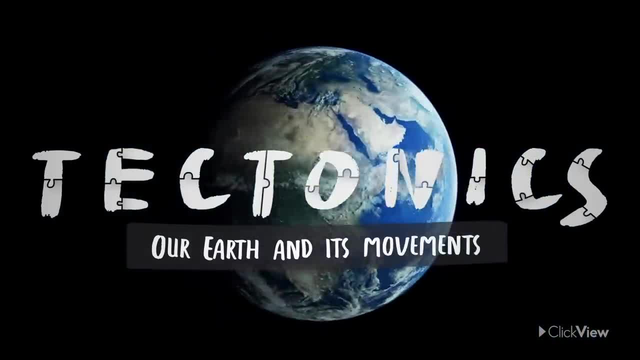 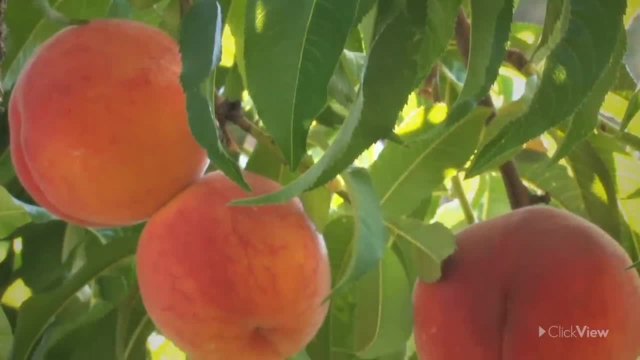 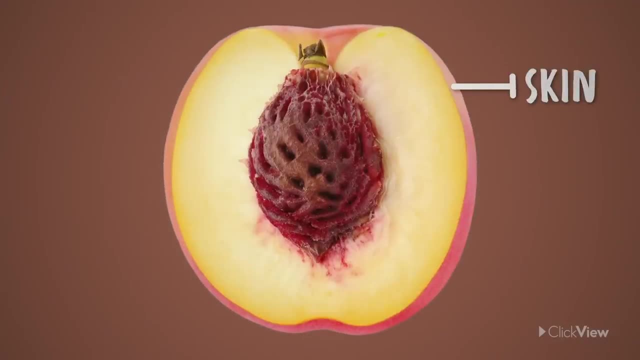 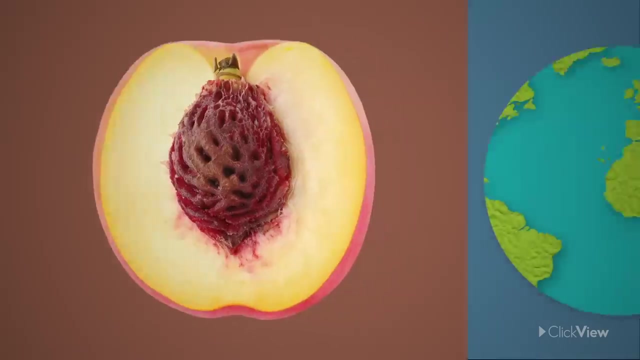 To get an idea of how much of the Earth is crust, take a look at this peach. A peach has three layers: A thin, hard skin on the outside, a thick layer of yellow flesh and a stone on the inside. Like this peach, Earth is also made up of several layers. The 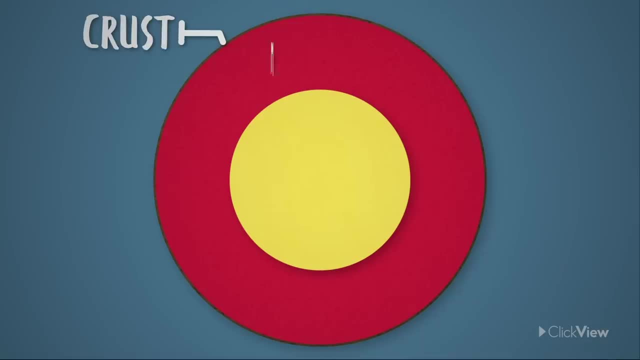 Earth is made up of several layers. The Earth is made up of several layers: The crust, the mantle and the core. Can you see how thin the crust is compared to the rest of Earth's layers? Under the crust lies a semi-liquid mantle layer of molten magma. 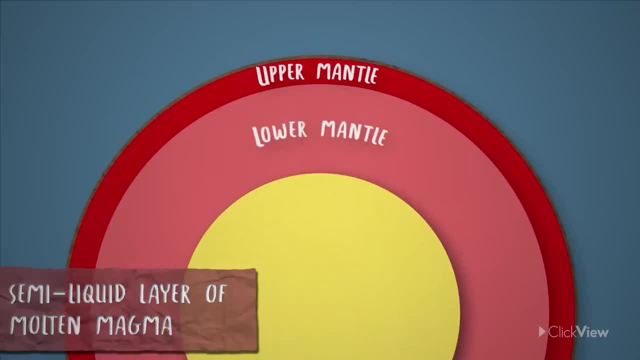 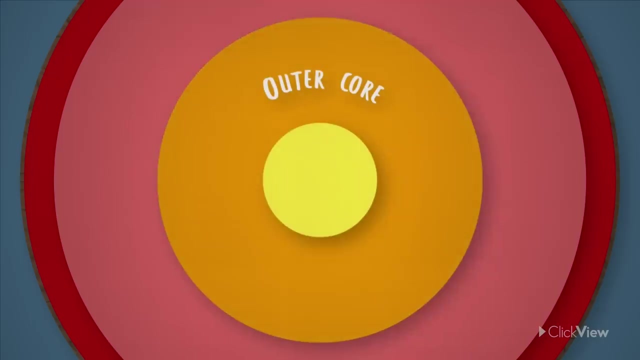 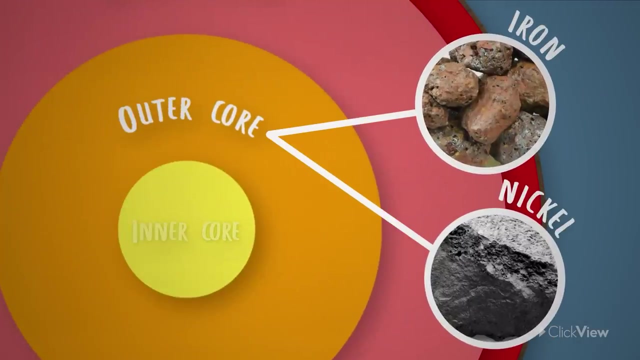 which can be divided into the upper mantle and the lower mantle. Together, the upper mantle and the crust are collectively known as the lithosphere. Below the mantle lies the core, which can also be divided into the outer core and inner core. The outer core is made of iron and nickel, But because temperatures are so high, 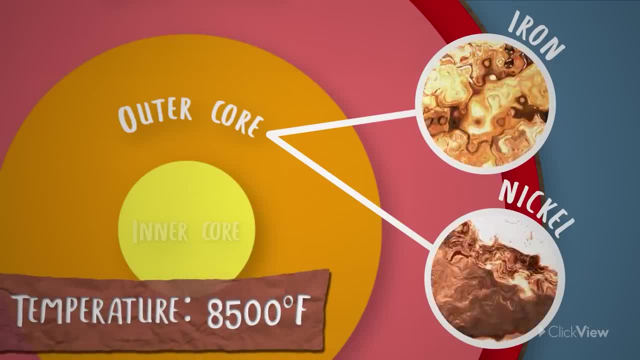 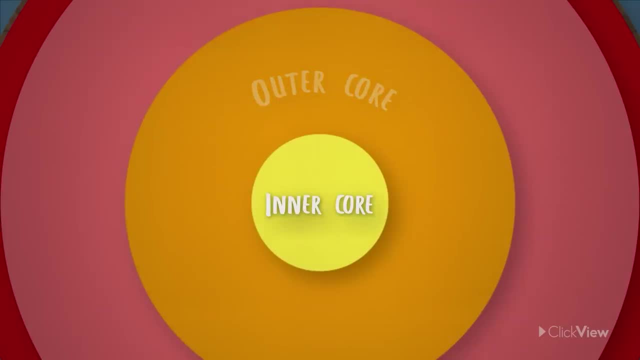 here you find these metals in their molten liquid form At the center of the Earth. beneath the outer core lies the inner core. This layer is a solid ball made of iron as well. The inner core is a huge metal ball made of iron, and 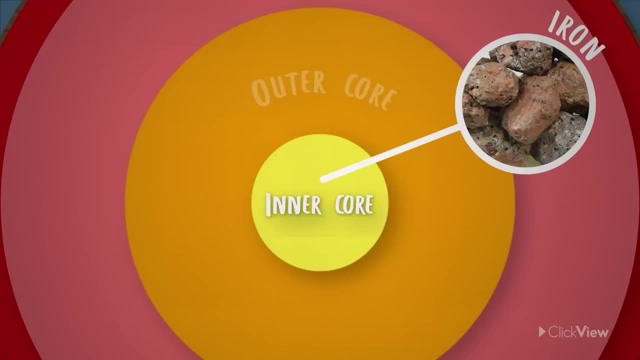 well, This is the hottest part of the Earth, with temperatures as high as the surface of the Sun. The inner core stays solid because Earth's gravity is so strong. the metals cannot melt, despite how hot it is. If you took a look at a world map, it would be easy to think that the Earth has always 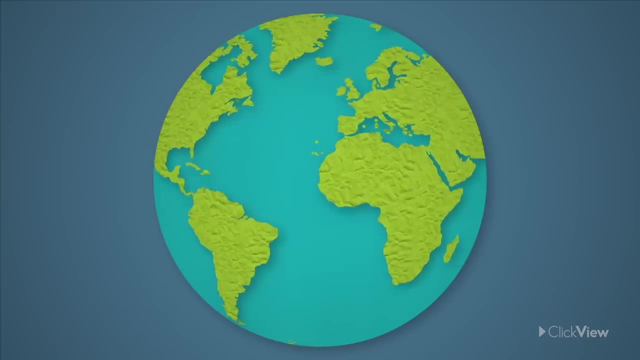 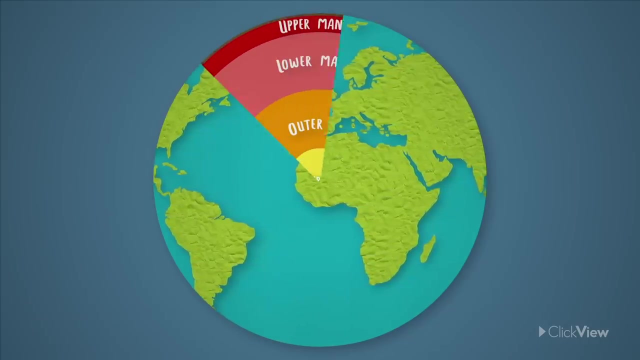 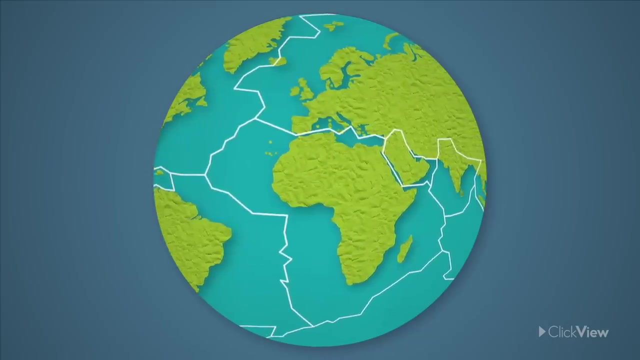 looked like this and always will. However, this is just how the Earth's surface looks currently, because it is changing all the time. Most of these changes happen in the lithosphere. Earth's lithosphere is divided into many tectonic plates that are different in shapes. 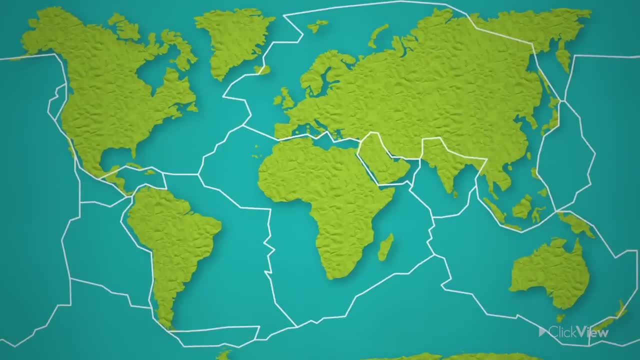 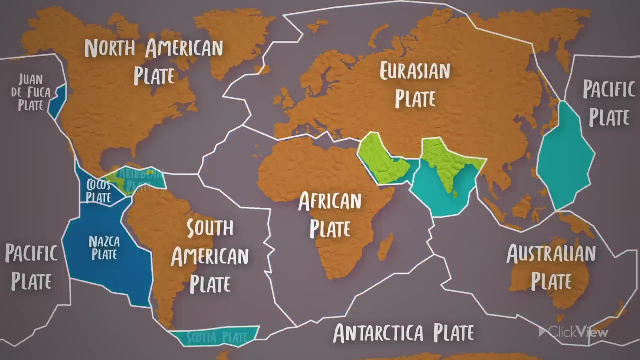 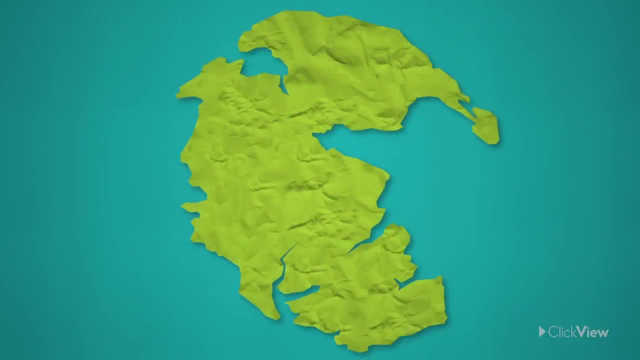 and sizes, but fit tightly together like a jigsaw puzzle. There are seven large key plates and several smaller plates, And are lands and oceans. Did you know that all of the continents that we know today once formed a single supercontinent? This supercontinent existed 335 million years ago and we call it Pangea. 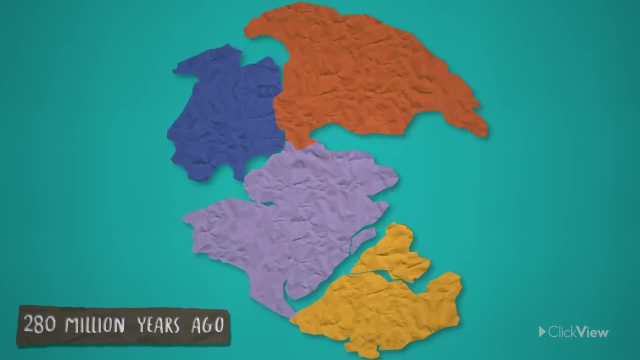 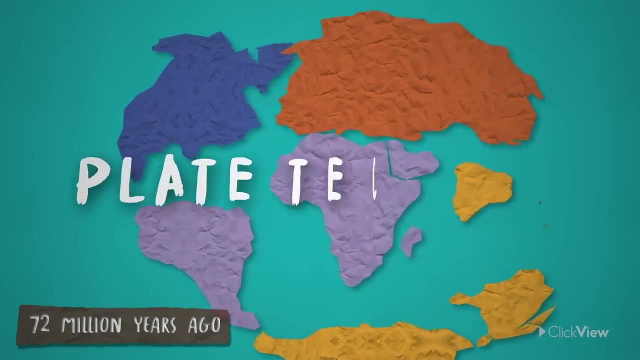 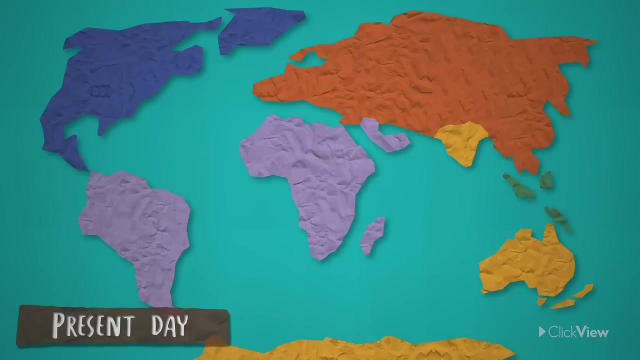 Over millions of years, the tectonic plates which hold the continents moved around, smashing into each other and then pulling apart. This process is called plating. This process is called plating. This process is called plate tectonics, but is sometimes also known as continental drift. 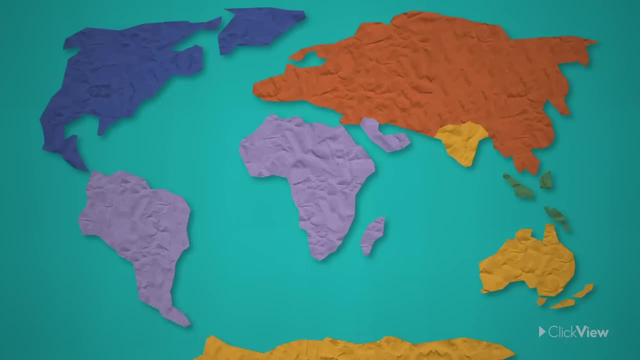 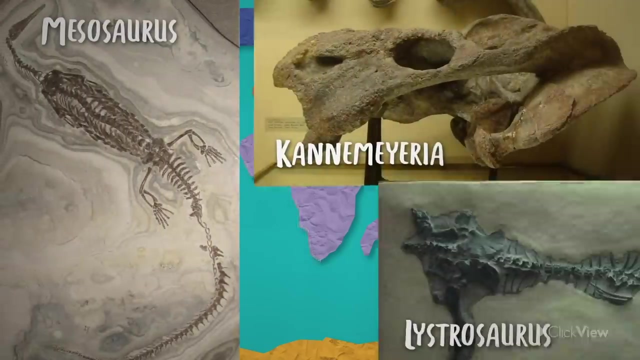 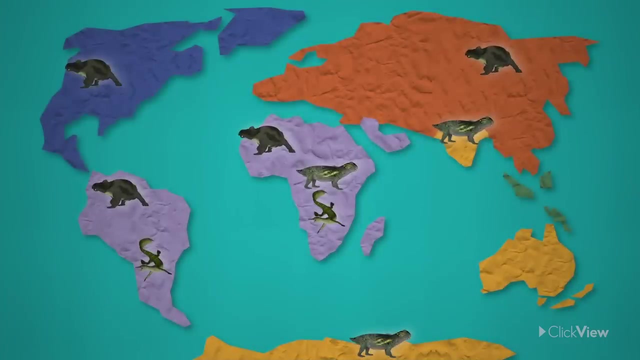 If you look closely, you can see where some of the edges of the continents line up, like the edges of Africa and South America. Fossils of animals that couldn't swim or fly have been found on different continents, providing further evidence that all the continents were previously connected. 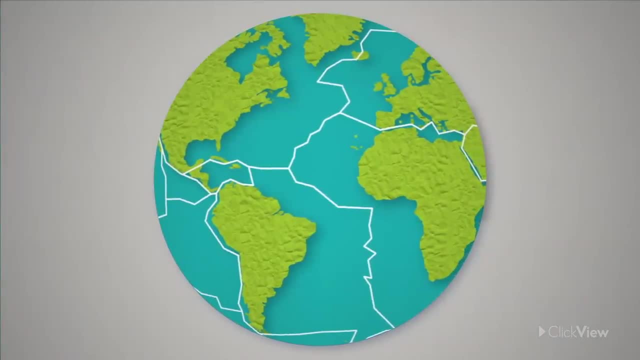 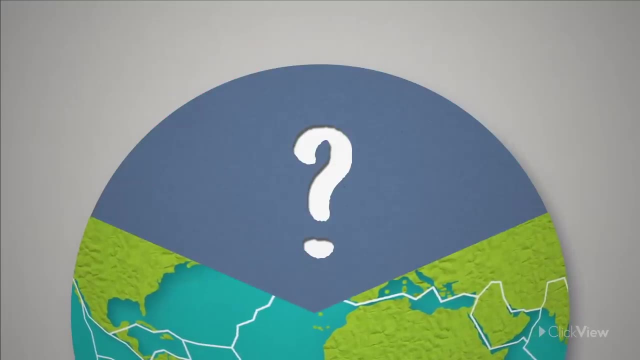 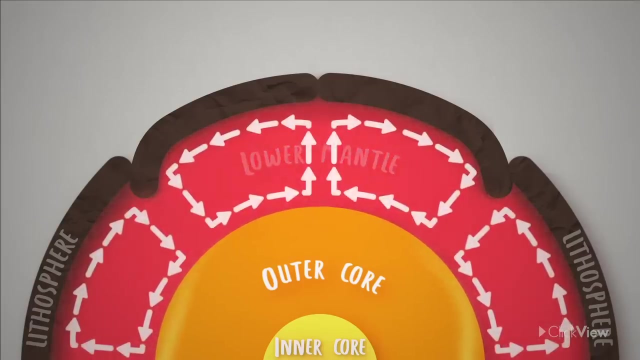 So how did the plates manage to move the continents to where they are today? To find out, we'll have to look at what lies under the plates. Within the Earth, there is tremendous heat and pressure, and this drives slow circular movements, called convection currents, within the mantle layer, which in turn cause the 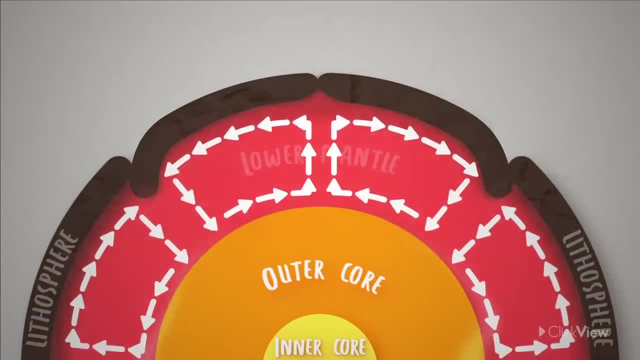 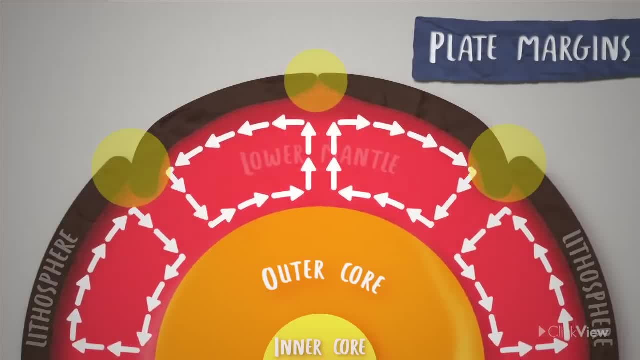 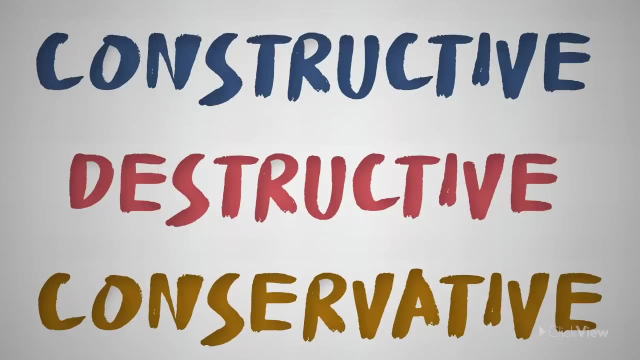 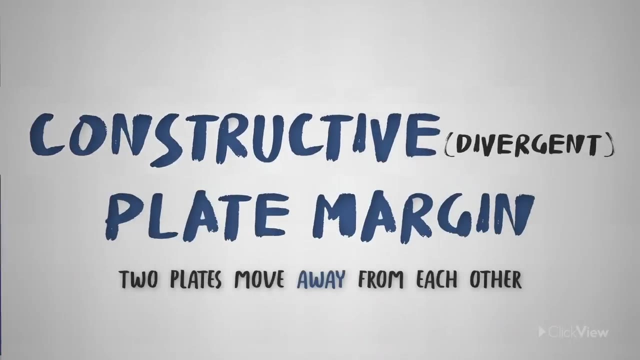 We can see the plates move between two plates at different speeds, which are known as plate margins. There are three types of plate margins, depending on what kind of movement occurs between the two interacting plates. At a constructive – or divergent – plate margin, two plates move away from each other.